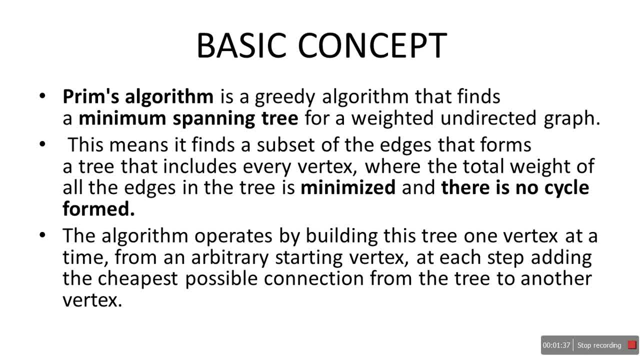 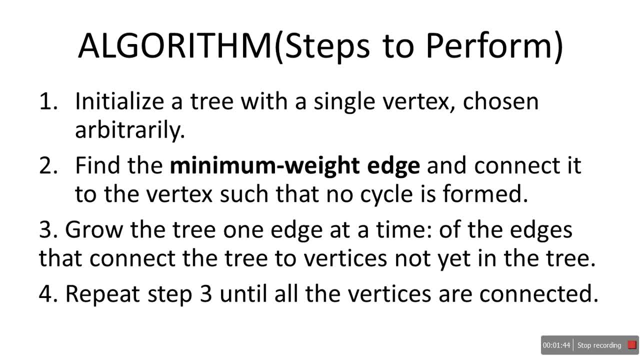 not previous vertex, but at least to the tree. okay, so we'll look at an example. you'll understand better. okay, so what is the algorithm or steps to perform? first one is initialize a tree with a single vertex chosen arbitrarily. mostly we'll choose a point or vertex where we have the 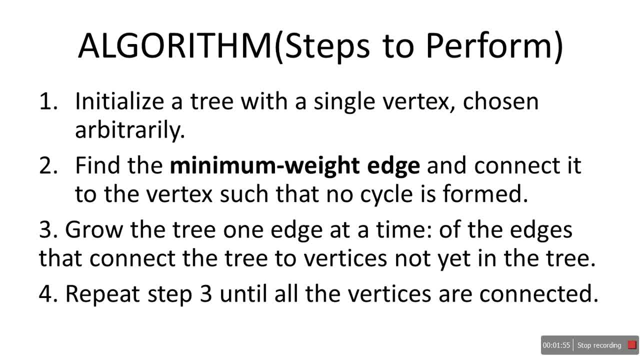 smallest edge connected to. okay, find the minimum weight is and connect it to the vertex such that no cycle is formed, okay. so this is step number two. third step is grow the tree, one edge at a time, of the edges that connect to the tree to vertices not yet in the tree. so basically you have. 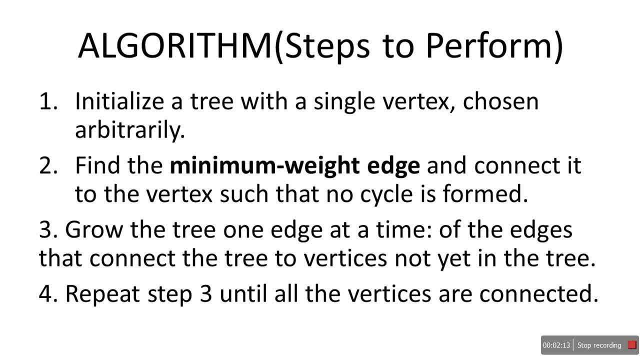 to connect it in such a way that the weight of that edge is small and it can be connected to one of the vertices that are present currently in the tree. okay, and repeat step 3 until all the vertexes unexpectedly move in. theول the vertices, the vertex package is shoot in one вами alt value. 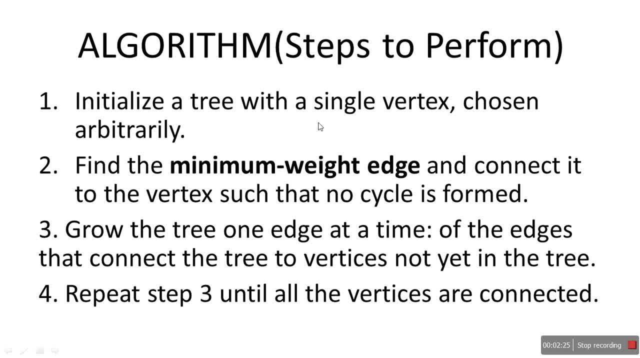 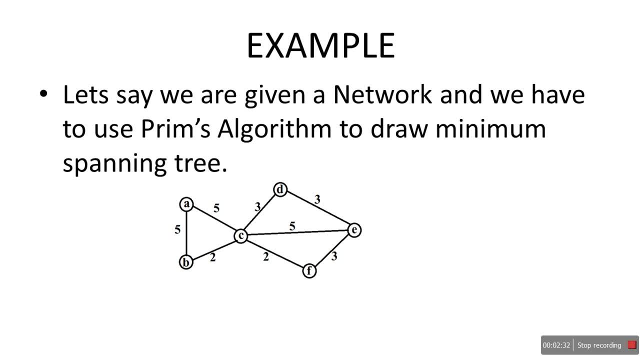 and repeat step three until all the vertices- click so to opaque, now drop or not, press enter- are connected. all right, so you do this until all the vertices are connected and we have a minimum spanning tree. all right, let's take a look at an example. let's say we are given a network. okay, this. 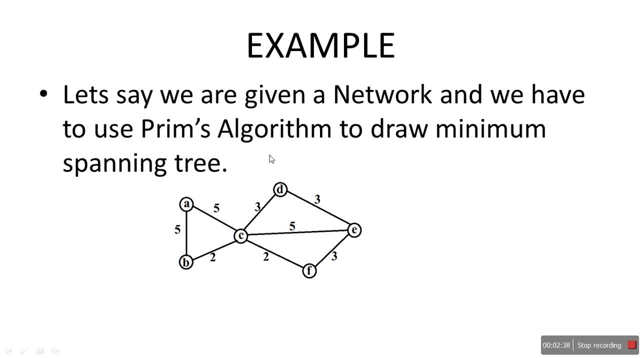 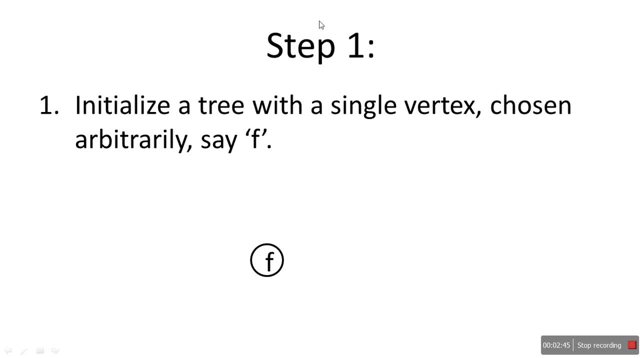 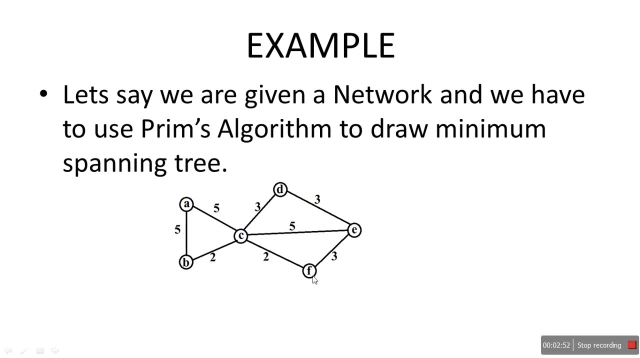 is the network that we are given and we have to use prims algorithm to draw minimum spanning tree. okay, so this is the network that we have given. so what we have to do, first step is step one: initialize a tree with a single vertex, so we'll choose, say f. okay, so we'll choose this vertex, f. 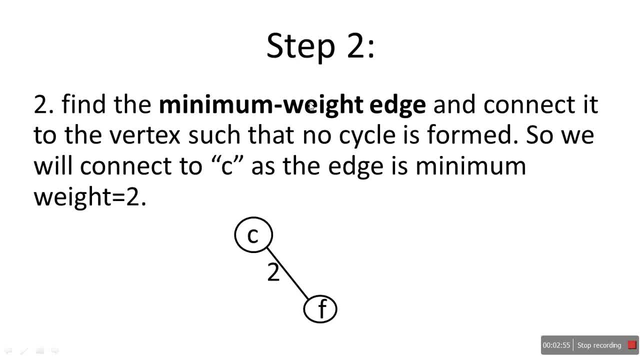 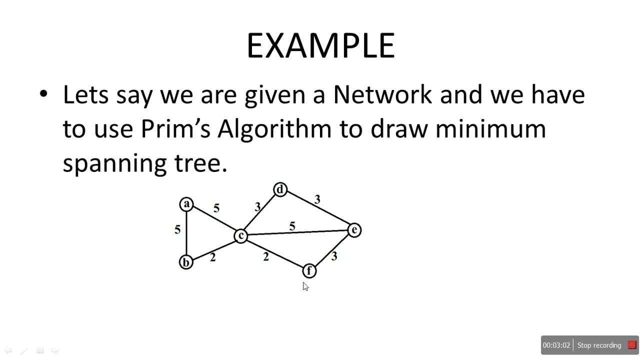 now what is step two? find a minimum weighted edge and connect it to the vertex such that no cycle is formed. okay, so, for example, we have taken f. now there are two edges connected to f. this one, f to c and f to e. f to c has weight equal to two. f to e has weight equal to three. so which is the minimum? 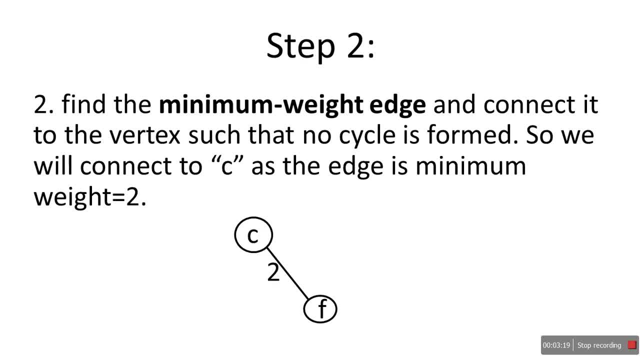 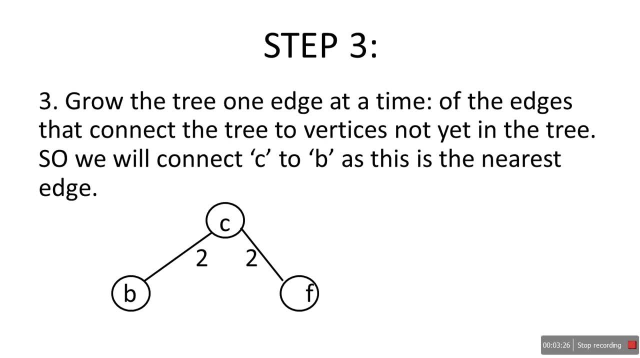 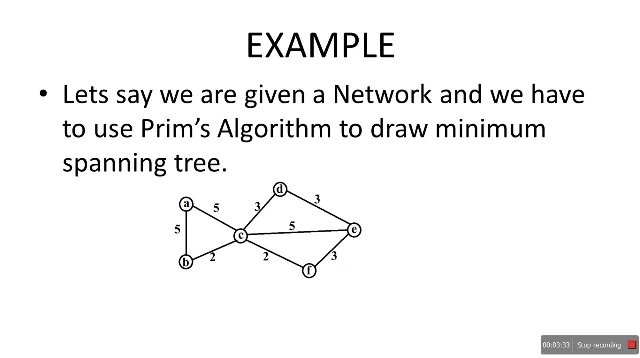 one, f to c. okay, so we'll add this edge now, because this is the minimum weight, equal to two. all right, step three is grow the tree one edge at a time of the edges that connect to the tree. two vertices not yet in the tree. so we connect c to b. why, as you can see now, we have 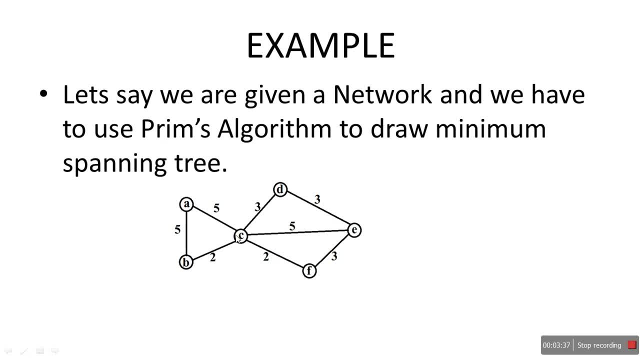 two vertices: okay, f and c. okay, c is connected to three, phi and two. so that is, c is connected to d, a and b and f. okay, and f is connected to e and c. out of all this, which is the minimum weight c to b, so we'll add that next, which next edge, which is connected to the tree, or at least one. 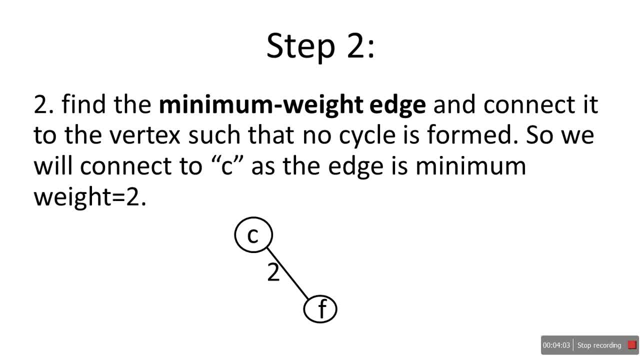 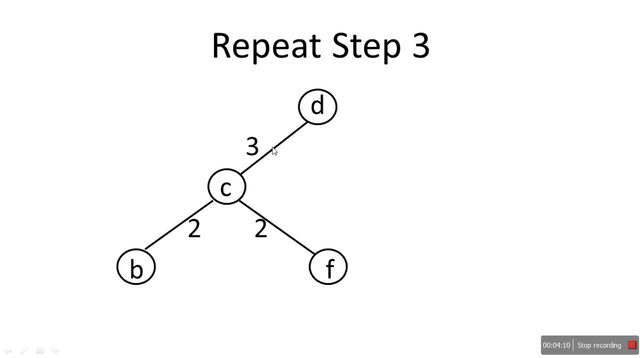 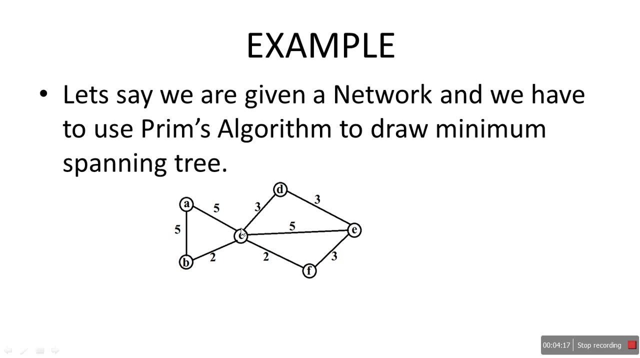 vertex is connected and it is having the minimum weight among them. so we'll add c to b. okay, now we'll repeat the step three. the next one will be c to d, or it can be f to e, also anyone. you can choose anyone, because the weight is equal: c, c to d or f to e. okay, so you can choose any edge. 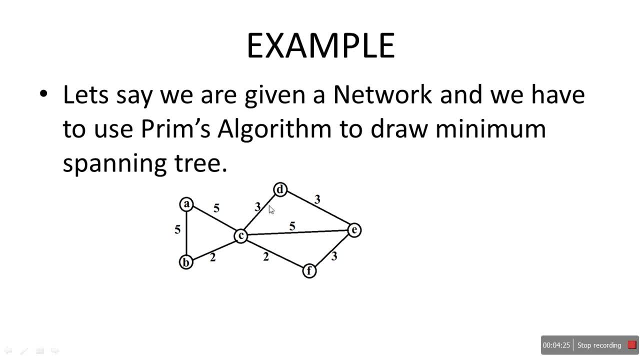 when they're equal. so we'll choose c to d. okay. now next step would be again finding the edge which is having the minimum weight. now, which edges are left? this one: c to a, a to b and d to e. okay, and also c to e is left. okay, but we don't want to do c to e because it will form a cycle between: 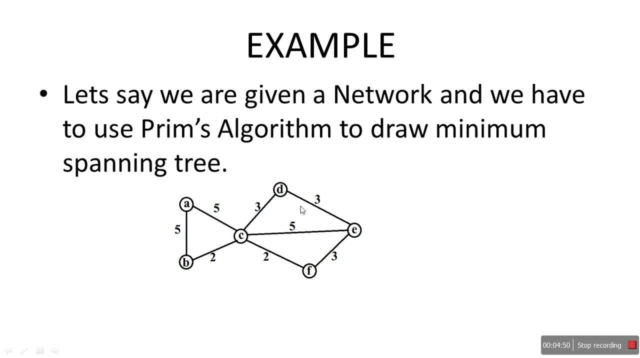 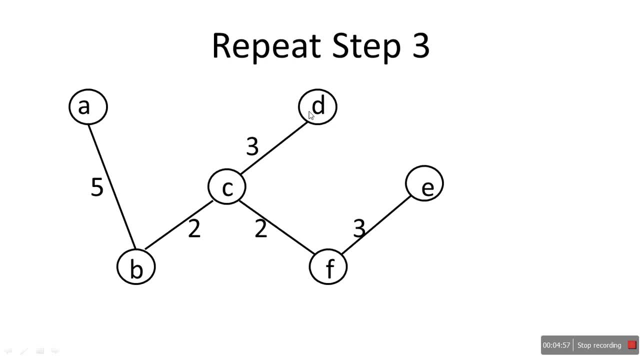 this three points, all right. so what we'll do? we'll add d to e because it is having the minimum weight. that is three. okay, yeah, all right, since we had chosen yeah, d, not d to e, d to e will also make a cycle, so we are not doing d to e. yeah, we are connecting. 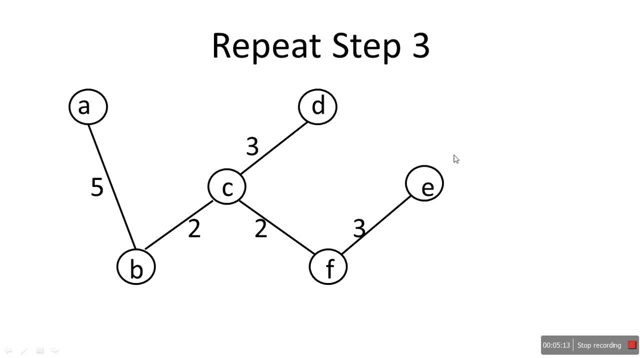 f to e over here, because it is also having weight equal to three. all right, next step, we'll add b to a, because that is the only point left which is unconnected, you can see over here. after over here, we'll add d, then from f to e, because it is having weight. 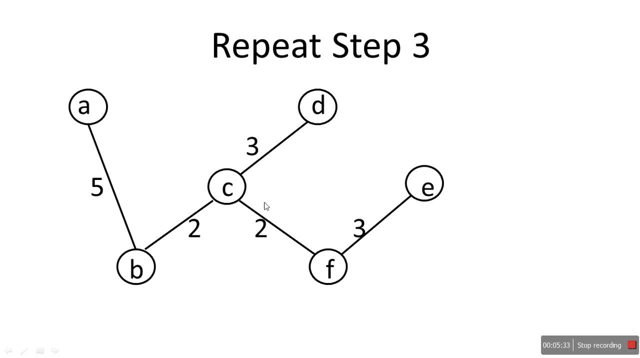 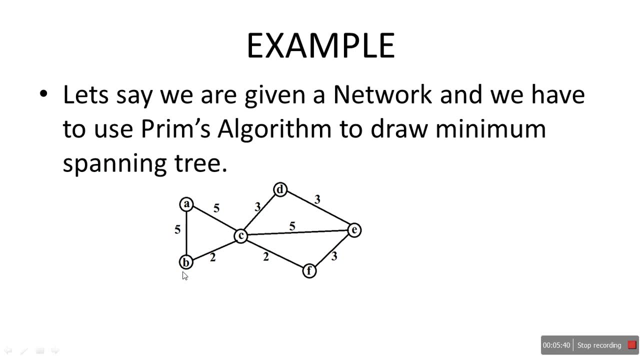 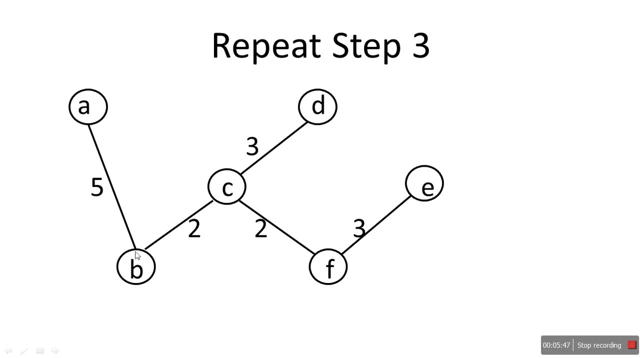 equal to three, and again after that. only a is unconnected to the whole tree. so what we'll do? we'll connect a anyway. a can be connected in either way, from c to a or b to a. both the weights are equal. so we choose c to b to a, all right, so we get b to a. that is equal to weight, equal to.